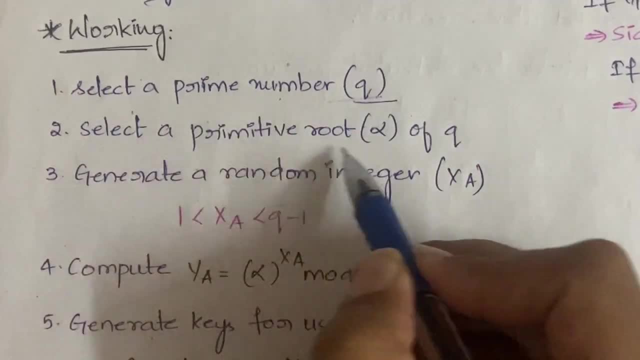 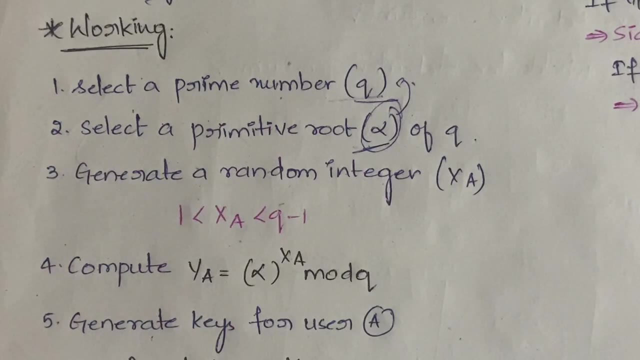 a prime number, a random prime number you have to select. and then you need to select a primitive root of q. Primitive root is denoted by alpha, So alpha has to be primitive root for q. So in order to understand what this primitive root is, you need to watch that Diffie-Hellman video. 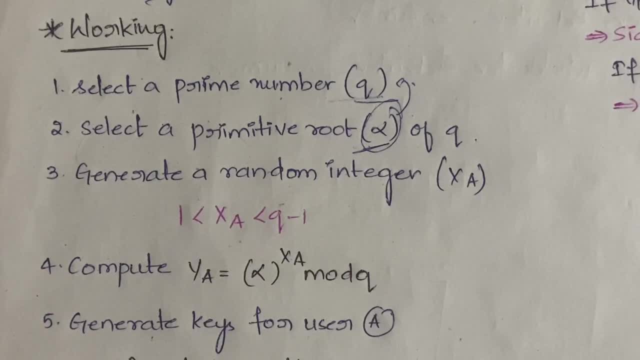 That is why I said you to watch that video Right. then you need to select the primitive root, Done. Next, what you have to do is you need to generate a random number. That is, you need to, like you know, you have to pick up a random number so that that number- random number- is denoted by xa. 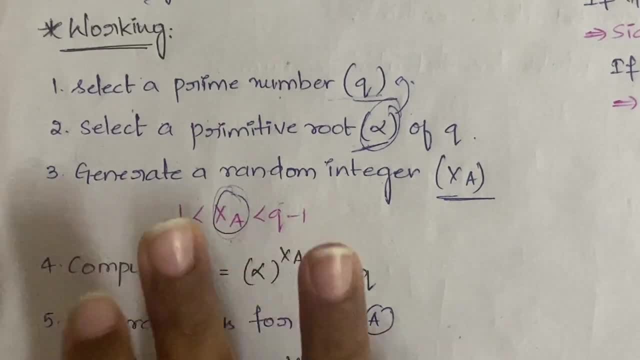 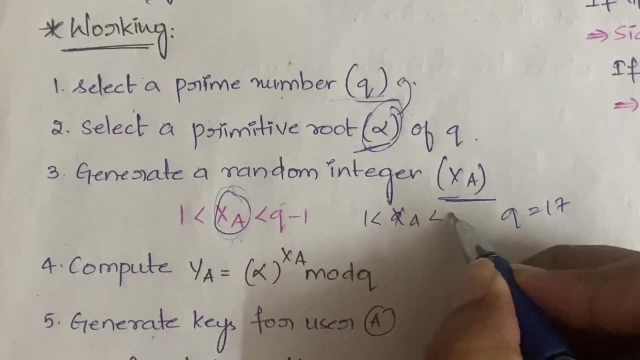 and that xa lies between 1 to q minus 1.. If you selected q as 17, then the xa should be between 1 to 16. right Between 1 to 16 you need to select xa. Got it? Next you need to compute ya After you. 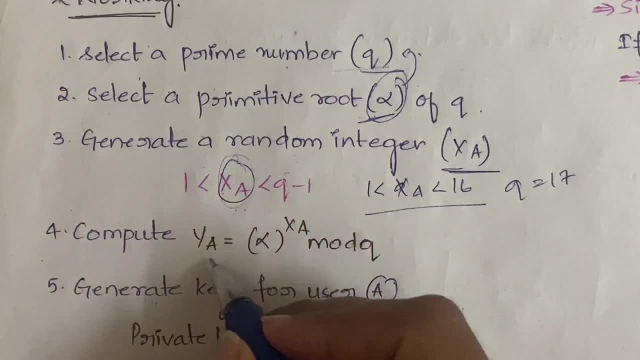 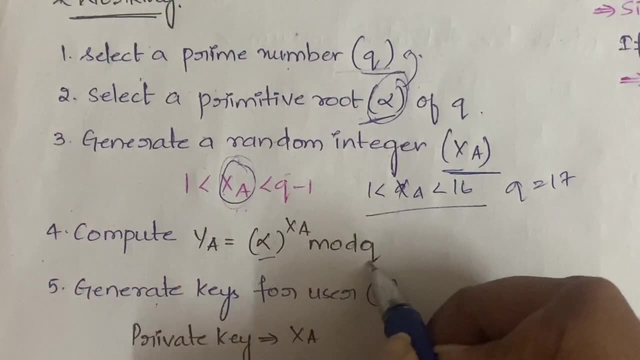 assume xa. you have to compute ya. How you will compute ya? ya is equal to alpha power xa mod q. What is alpha Primitive root? xa is a number which you have assumed and q is a prime number that you have assumed, Got it? So you need to collect, you need to compute ya Right. next, you need to generate. 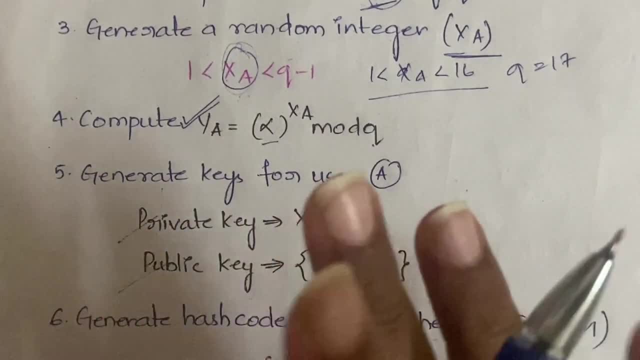 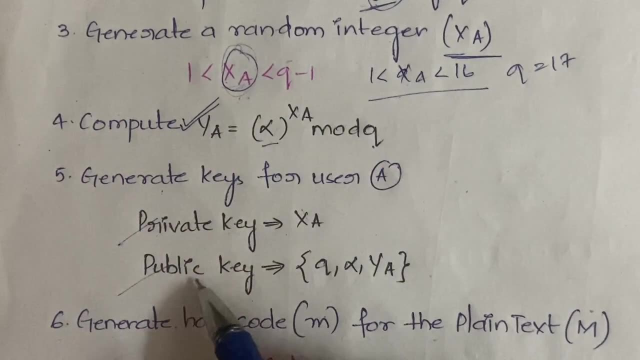 the keys You need to generate the private and public key for user a Right, so private key for user a Right. you have assumed some number, xa here, Right, so direct. that number will be. Next public key will be q comma, alpha comma. ya, Right, don't get confused When I explain with example. 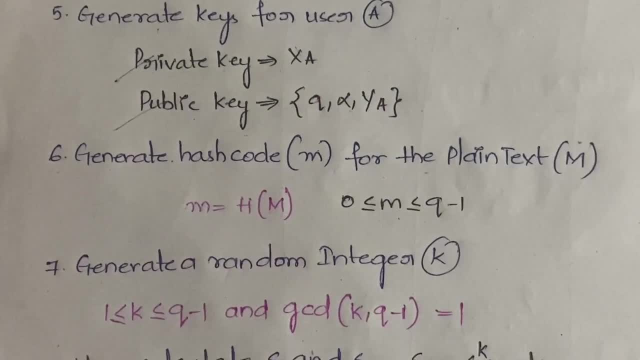 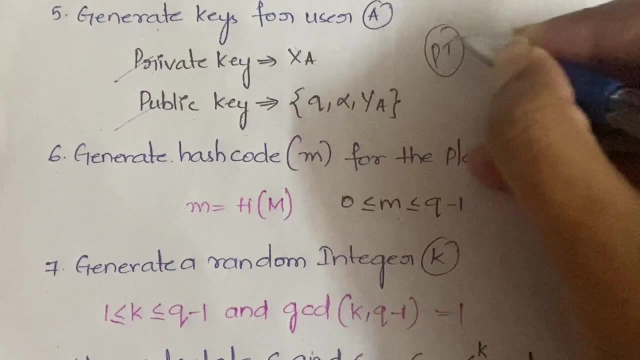 you will get a clarity Right now. you need to generate a hash code that also you can assume on your own for the plain text. Actually, we have the plain text Right. we have the plain text For plain text. whenever we do the hashing, we get the hash code Right. so, but here we are directly. 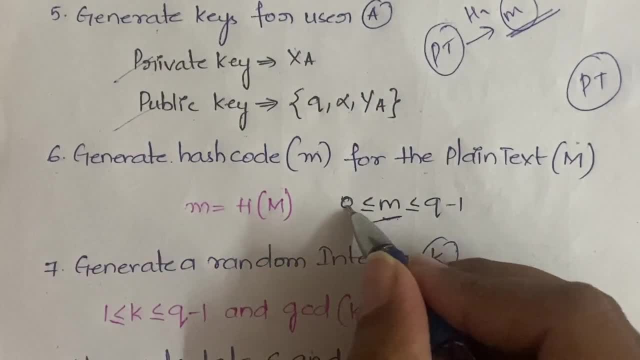 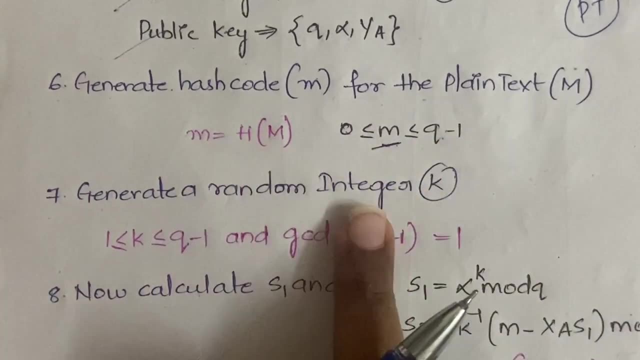 assuming something. and that hash code also has to be between 0 to q minus 1.. Right, so you need to calculate q minus 1 again. Okay, next, generate a random integer k. Now again, you need to generate another random integer k in such a way that one is less than or equal to. k is less than or equal. 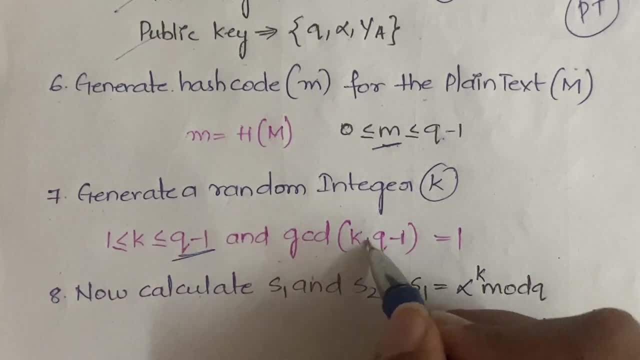 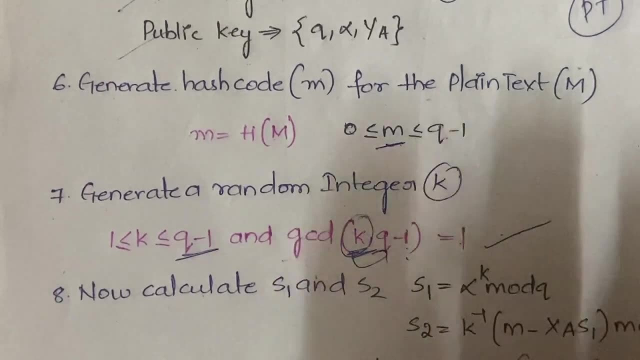 to q minus 1.. Again, q minus 1 and gcd of k comma, q minus 1, should be equal to 1.. So whatever number you are assuming, gcd of this number and q minus 1 should be equal to 1.. Got it Now in the last in. 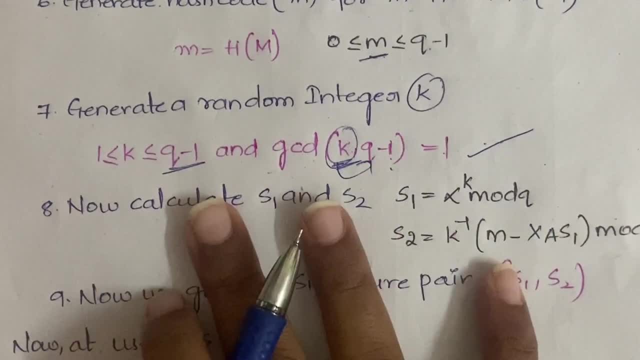 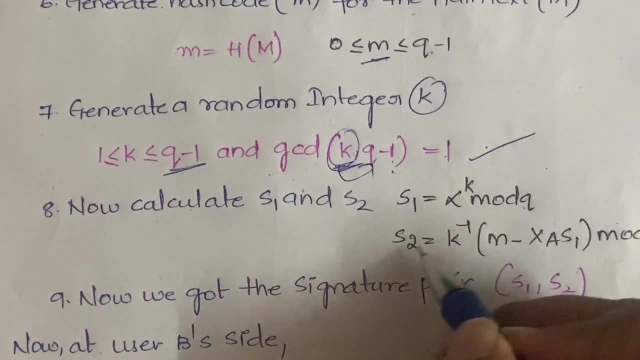 the next step. what you have to do is you need to calculate s1 and s2.. So what is this s1 and s2.? I will let you know. Signature pair: S1 will be equal to alpha power, k mod q, and s2 is equal to k. inverse into m, m is nothing but the. 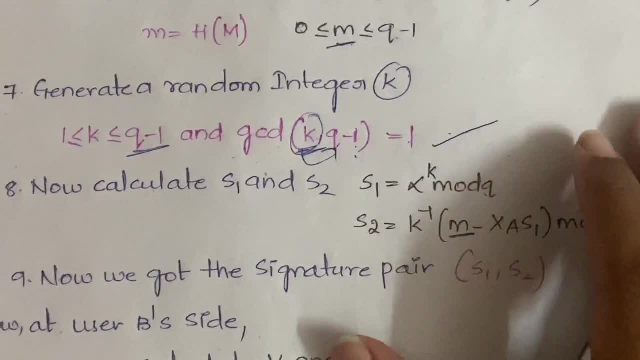 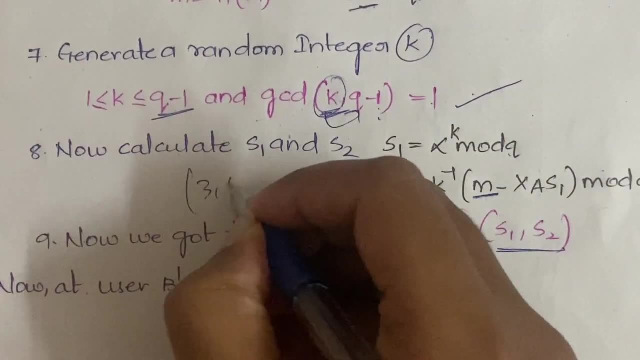 hash code minus xa. s1 mod q minus 1.. With example you will understand, Don't worry. Right now you will get the signature pair s1 comma s2.. Whatever values are generated, Suppose if you got 3 comma 4.. So you need to write 3 comma 4 as a signature pair. Got it Now. we got the signature pair Now. 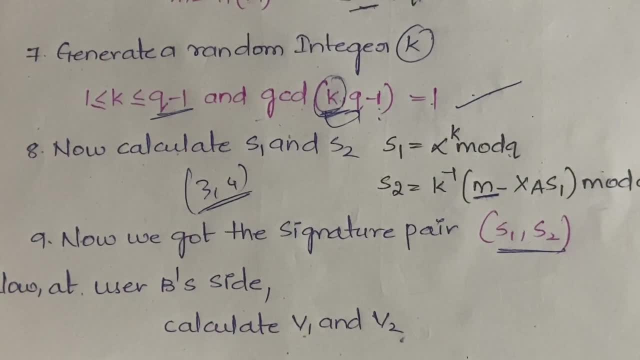 at user b side. User b side in the sense at the receiver's end. So till now, what we have done on the receiver side, what will happen? We need to calculate v1 and v2.. Right, So what is this v1 and? 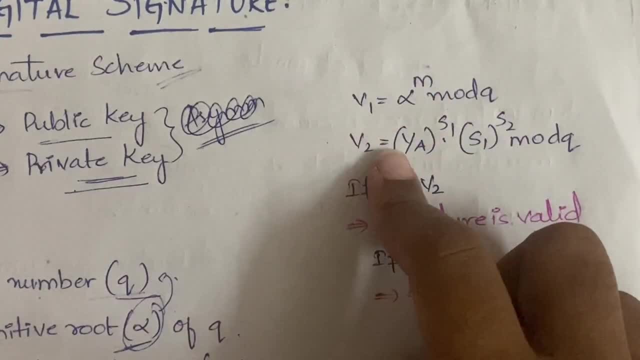 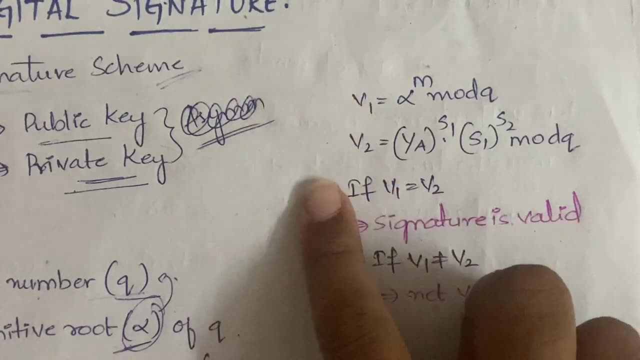 v2.. I'll tell you: v1 is equal to alpha power m mod q and v2 is equal to ya power s1 and s1 power s2 mod q. Right, You need to calculate v1 and v2.. If you get v1 and v2, both are equal. then the signature. 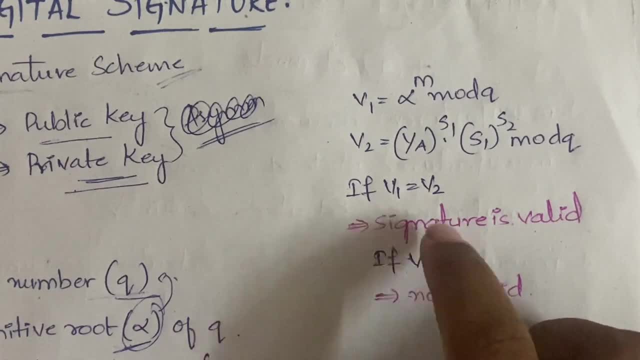 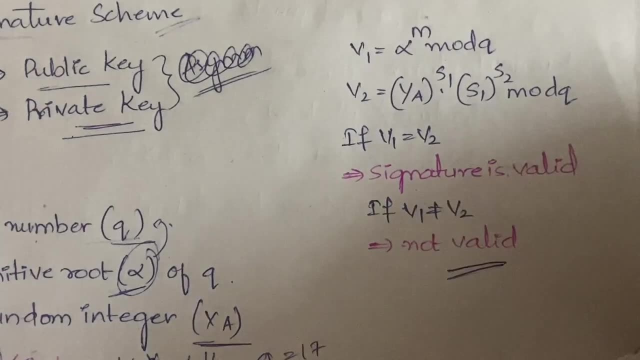 is said to be valid, Right? If the, if you know, v1 is not equal to v2, in that case the signature is not valid, Got it? So I'll explain you this with an example, Then you will understand It more clearly, Don't worry. So, coming to the example now, let us assume the values of q and. 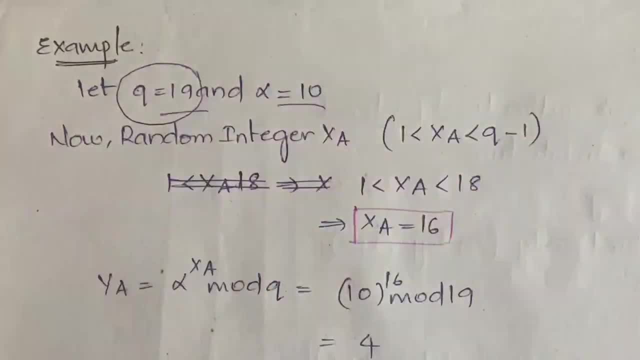 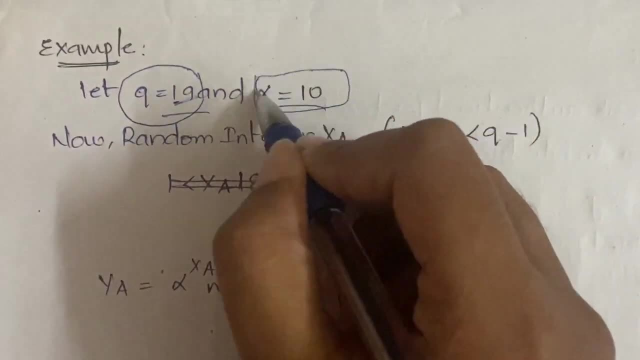 alpha initially. So we have to know, we have to first assume the value of q Right. q is equal to 19.. We have taken q is a prime number only Right. Now you have to calculate the value of alpha. Alpha is nothing but what the primitive root of q Right. So in order to understand what 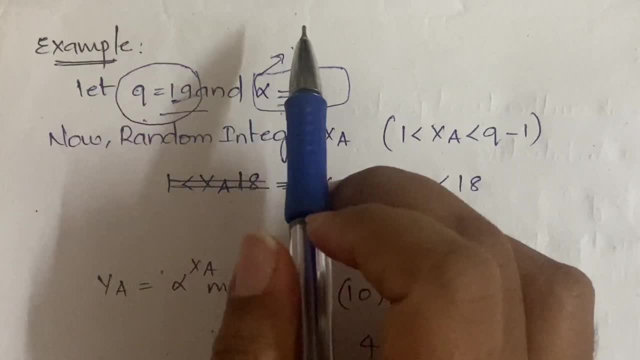 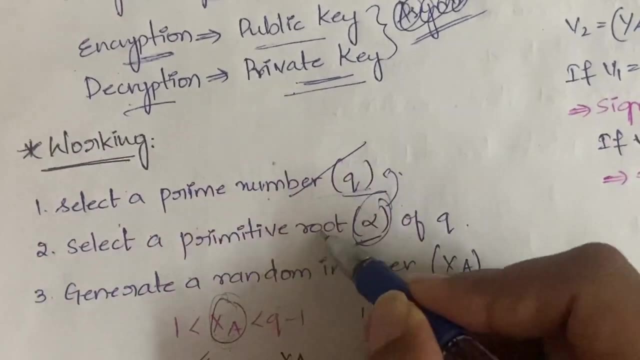 is primitive root. I you know, you watch that Diffie-Hellman key exchange algorithm video. you'll understand Now what you have to do in the second step, what you have to do. So here let us see: first number done, primitive root done and you have to generate a random integer such that it is less. 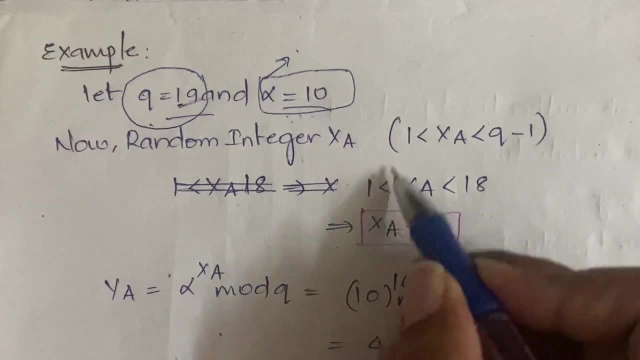 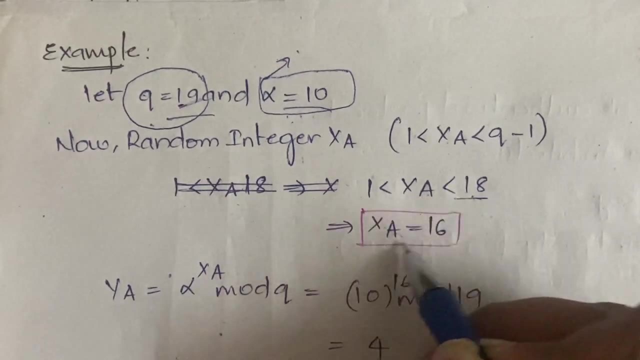 than q minus 1.. So you have taken it as: 1 is less than x, a is less than q minus 1.. Right q is 19.. So it should: 19 minus 1 is 18.. So 1 is less than x, a is less than 18, and we have assumed it as. 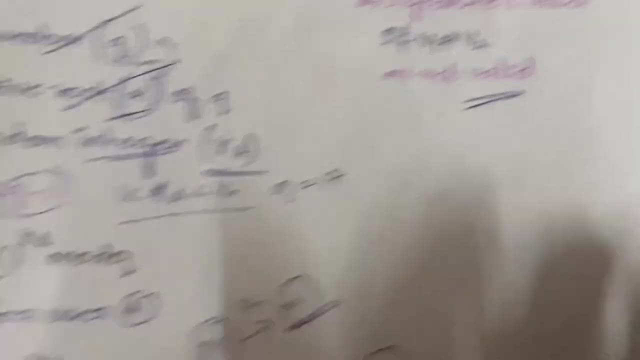 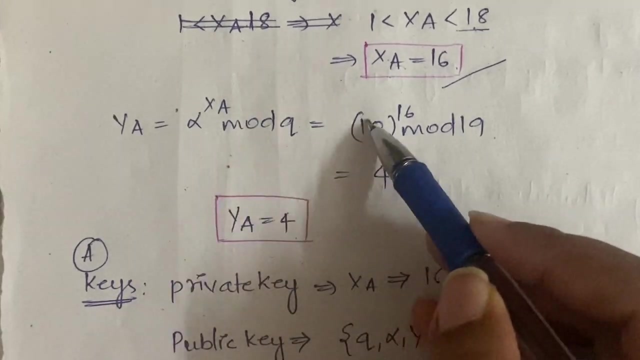 16.. Anything you can take Done Now. next step: what you have to do: x a done Now. you have to calculate the y a. y a is what alpha power, x a mod q, Right, So alpha is what 10? and. 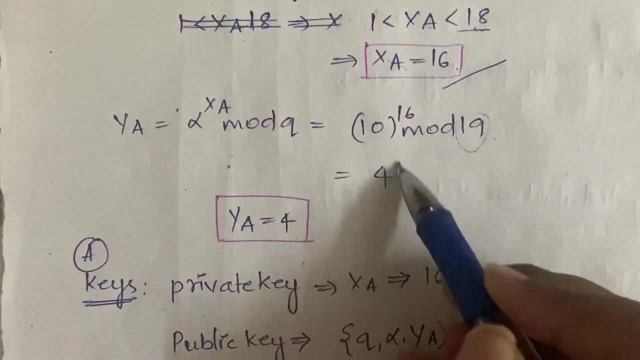 x a is 16 we got, and mod q is nothing but 19. we have assumed Right, You'll be getting 4.. So how you get 4 is you can use calculator, Since you are allowed to carry your calculator in your exam. 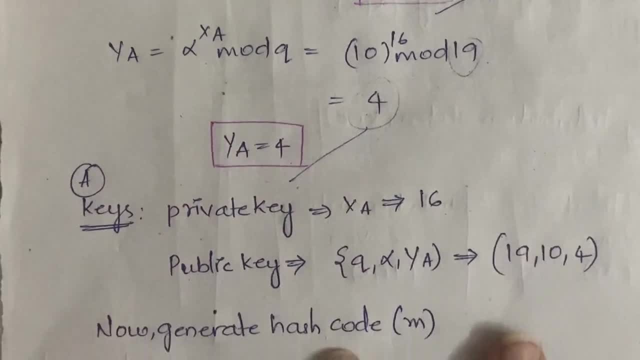 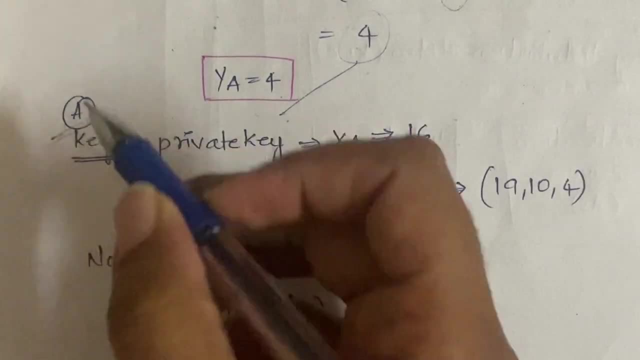 you can use the calculator. you'll get the value for this Done. Next, what you have to do, you need to generate the keys. The next step: generate keys for user a, So this is for user a. The keys of user a- private key and public key. So what is a private key? x a? So what is x? a? here we have got. 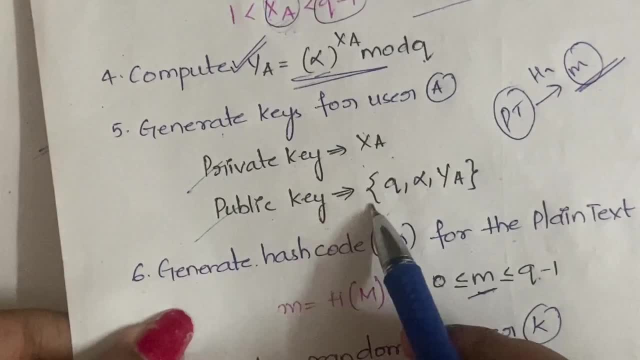 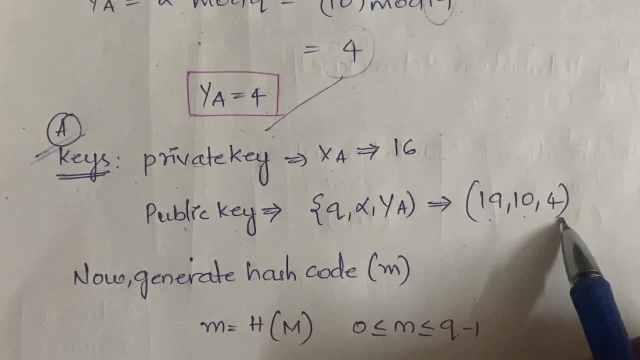 x a as 16.. So x, a will be equal to 16.. And what is a public key? Q comma, alpha comma, y a Right. So q we have assumed at 19, and alpha we got as 10 and y a we got as. 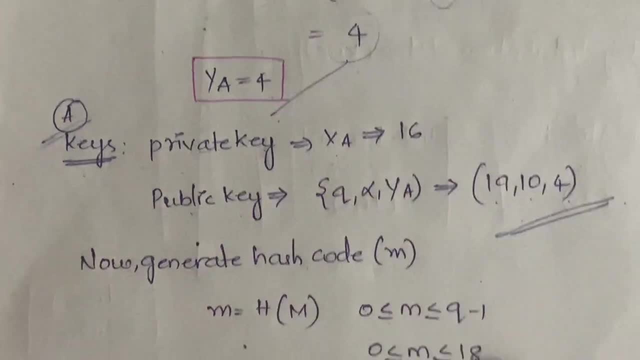 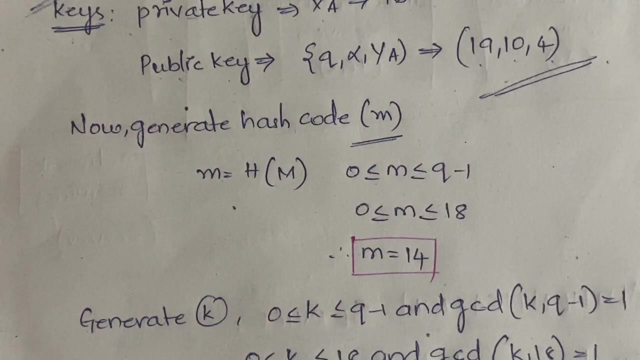 4 here Done, So public key and private key are generated, Done. Next you have to generate a hash code. OK, M. So for the plain text you need to generate the hash code, and we have directly taken the hash code as small m, So that also has should lie between 0 to q minus 1.. Right, So we have. 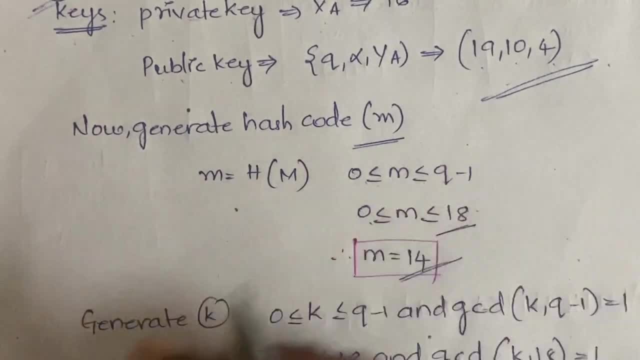 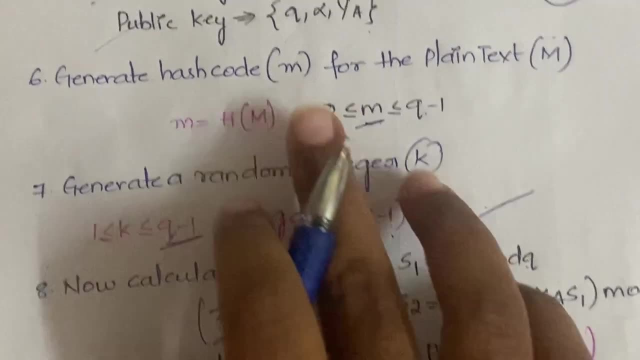 assumed it as 14.. q minus 1 is 18.. So 0 to 18, it can lie. We have taken it as 14. Done. Next, what you have to do: you need to generate. So hash code is done, Hash code is done, We are done. 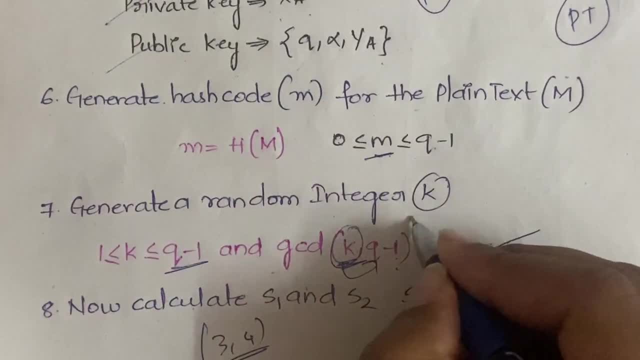 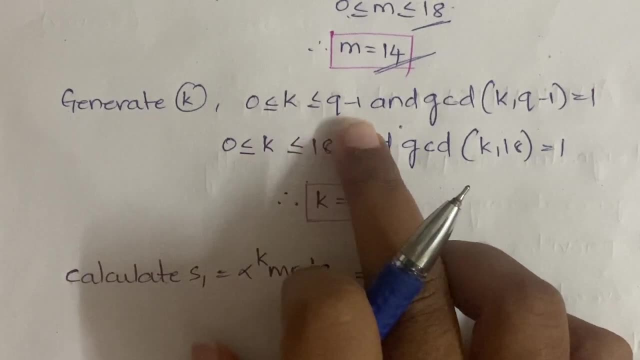 up to sixth step. Then what we are doing? we are generating a random integer, k And also k also has some constraints, Right? So let us see: So 0 is less than, k is less than or equal to q minus 1, and 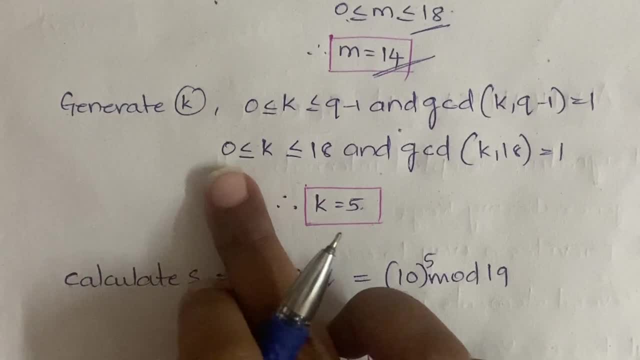 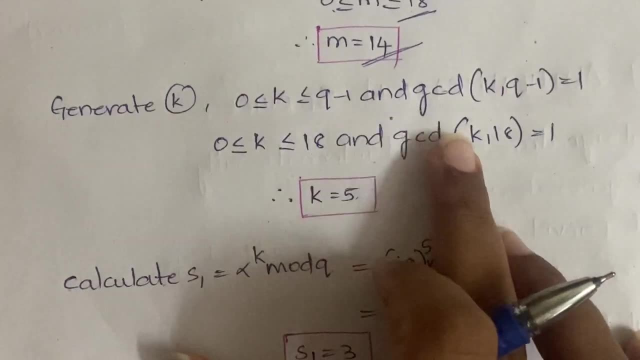 gcd of k comma q minus 1 should be equal to 0. So here 0 is less than or equal to k is less than or equal to 18, because q is 19, 19 minus 1 is 18 and gcd of again k comma 18 should be equal to 1.. So 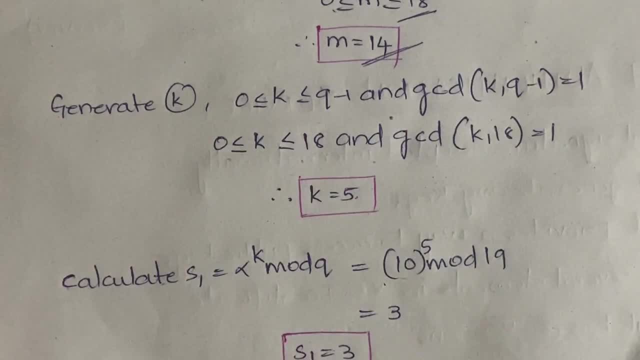 5 is lying between 0 and 18 and also gcd of 5 comma 18 is 1.. What is gcd, greatest common divisor, Right? So the common divisor for 5 and 18 is obviously 1, because they won't both together won't. 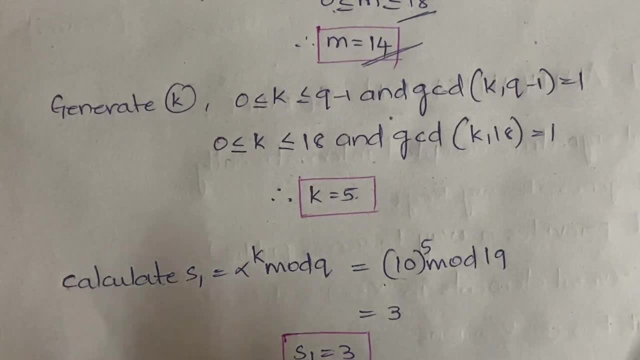 go in any table. Right, So it is 1.. So we have assumed the value of k as 5. Done. Now, after getting the value of k, what we are supposed to do? we need to calculate s1 and s2 and for s1 and s2, 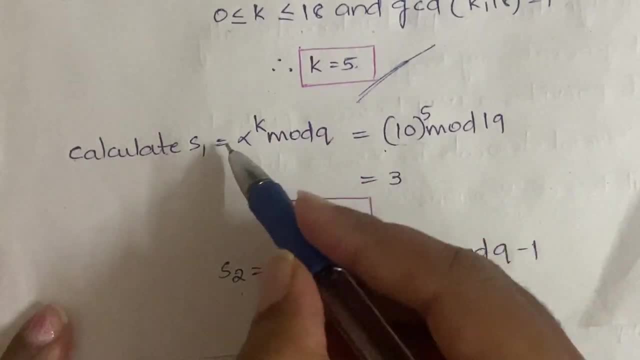 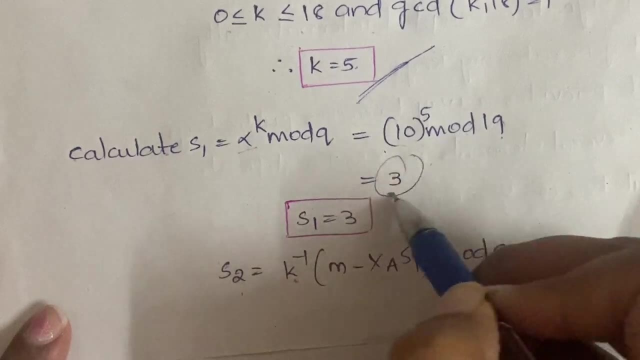 we have formless. So now I'll tell you, be careful. So s1 is easy: Alpha power, k mod q, which is equal to 0, and k we have generated as 5, then mod 19, we get 3. again, use the calculator, you'll get it So. 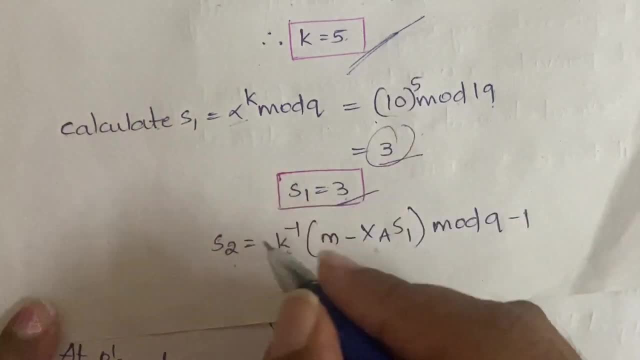 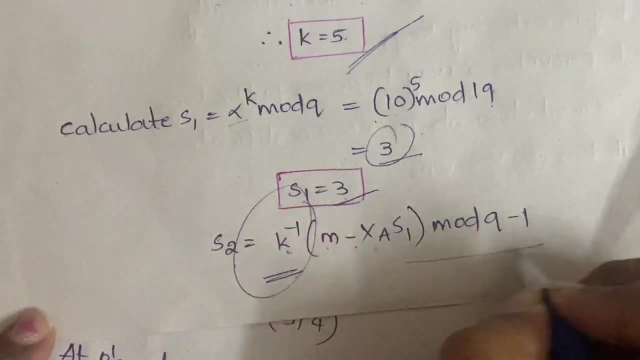 s1, 3. we got it. Now we have to calculate s2 for s2. what we need? we need k inverse. and how to get this k inverse. I'll tell you: k inverse m into m minus x is 1 mod q minus 1.. So how to calculate? 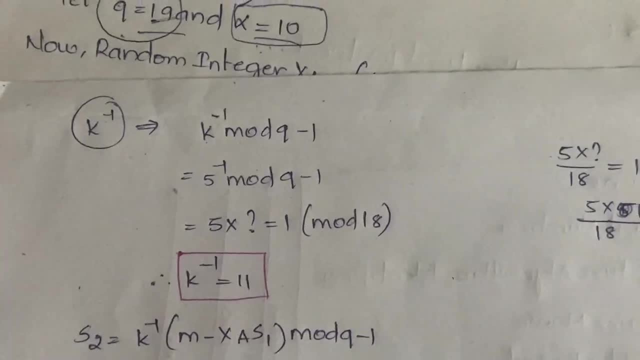 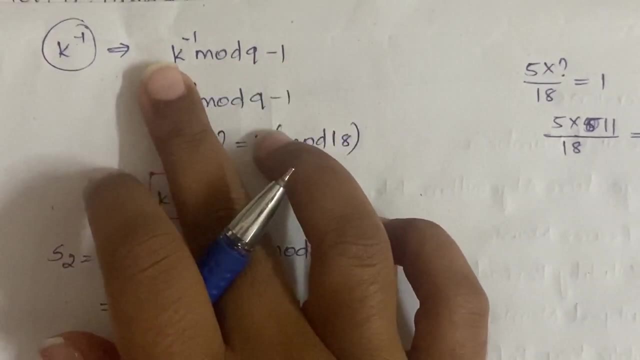 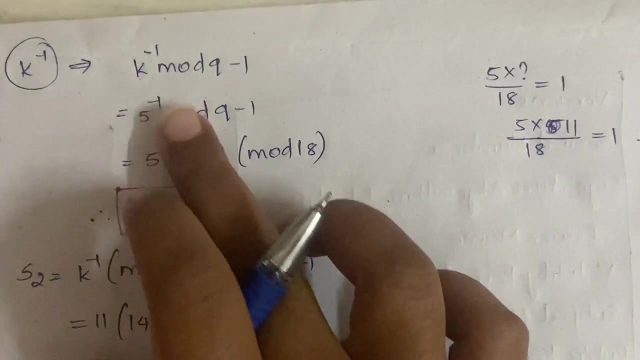 this k inverse. I'll tell you. So see, in this paper. yeah, k inverse mod q minus 1, you have to find out, right. So k is nothing but what. we got the value of k as 5 here. We got the value of k as 5, right, So it is 5. inverse mod q minus 1 is nothing but what, 18.. So 5. 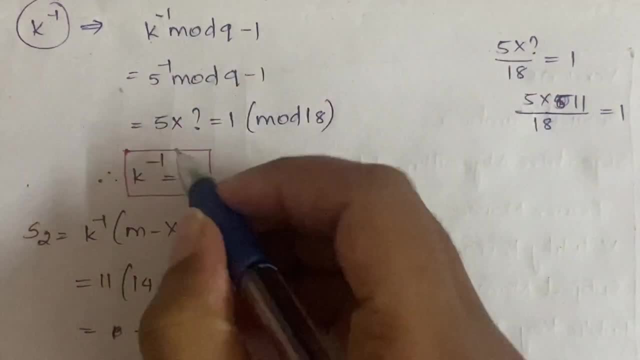 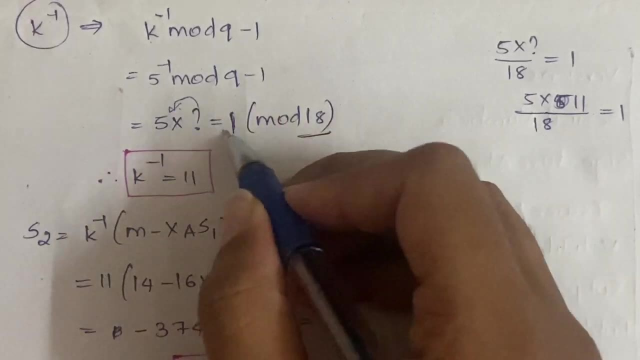 inverse mod q minus 1 is nothing but what you have to multiply to 5 in order to get 1 when you divide it with 18.. Got it 1 mod 18, you need to get Which number has to be multiplied here when. 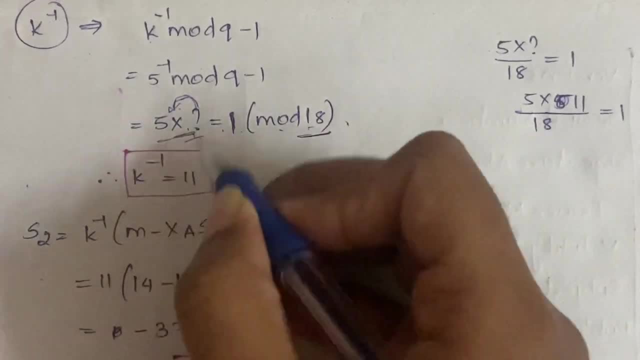 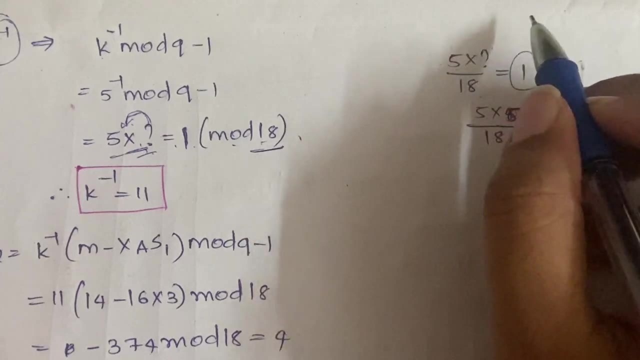 you so that you get 1 when this number is divided by 18.. Right, So 15 into what gives by 18.. Will give you 1. So 15, sorry, not 15, I'm sorry. 5.. So 5 into 11 is what 55, right? And what is 18 3's? 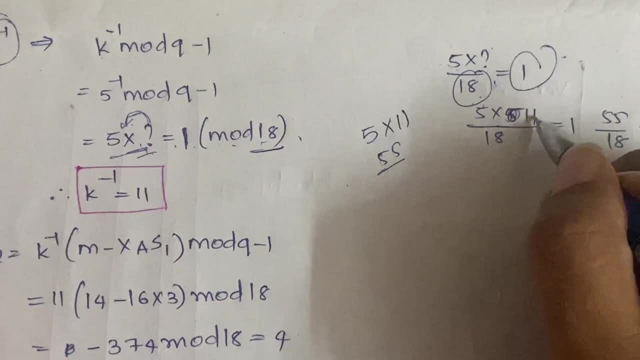 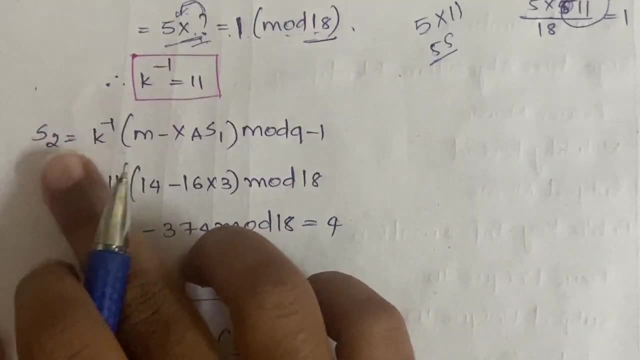 are it's 54. So the remainder is 1.. So you get the remainder as 1 when you take 11.. So therefore k inverse will be equal to 11.. Got it Next s2. s2 is equal to k. inverse m minus x is 1 mod q minus 1. 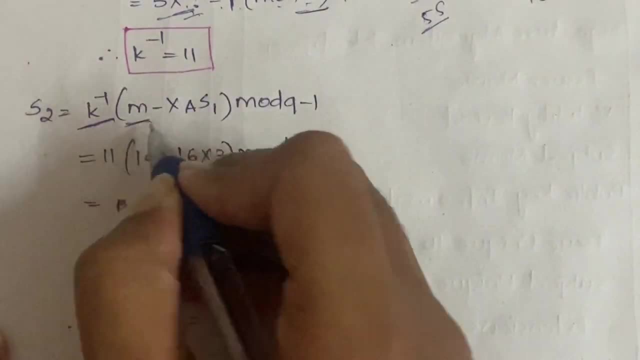 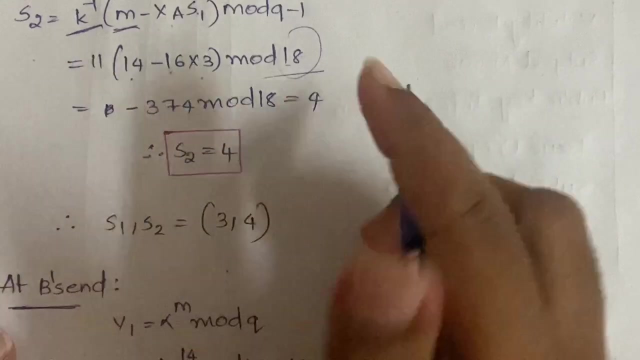 right. So we got the value of k inverse 11. m is 14. we have assumed x is 16, s1 is 3. we got mod. q minus 1 is nothing but mod 18.. Once you do this modulus, you'll be getting s2 as 4.. Done So. 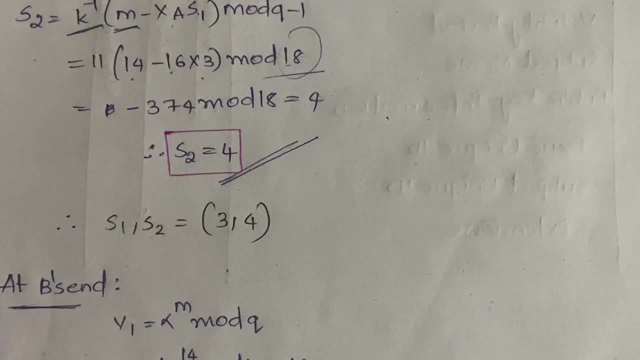 now you got s1 and s2.. Now you what you have to do after you got s1 and after you get s1 and s2, you have to generate the signature pair. Signature pair is nothing but simply s1 comma, s2 in form.